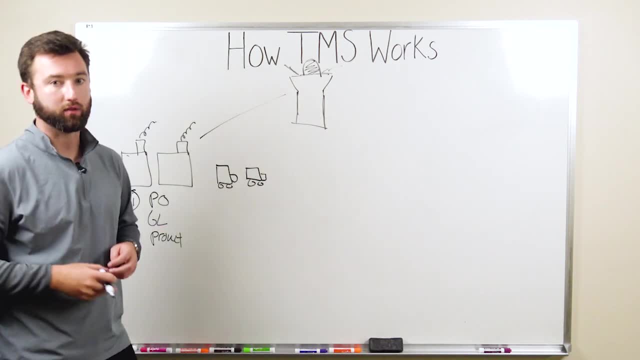 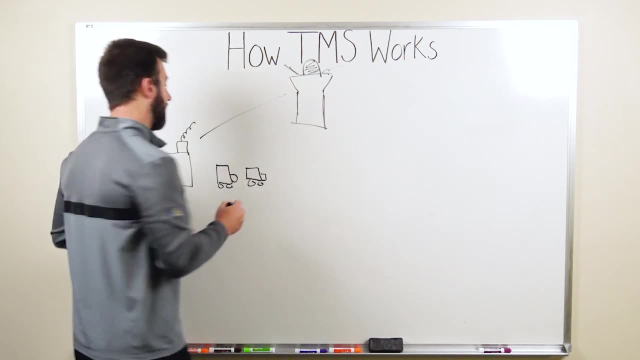 you're a large shipper, you probably have relationships with many carriers. You have LTL carriers, you could have parcel carriers, you could even have air and ocean carriers in the right TMS, And so all of that information is going to be. 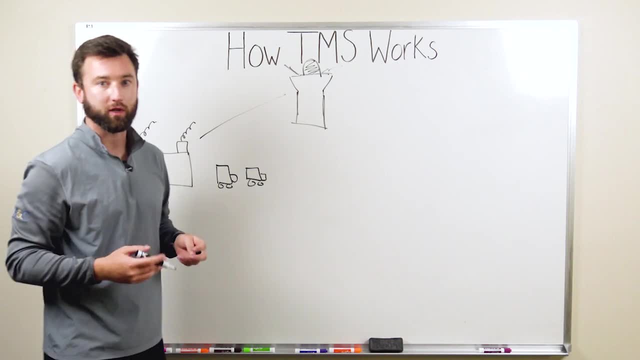 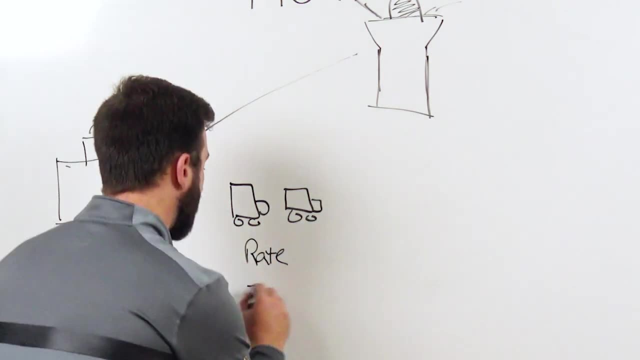 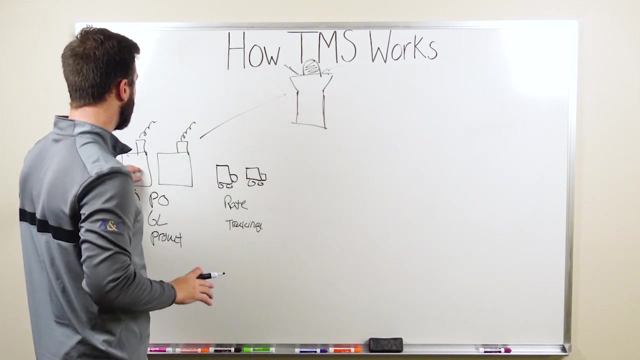 also be stored in the TMS. So what are some types of information that you might want to have? Well rates, What does it cost to move the goods? Tracking Where are my goods? right, As these goods say, move between your. 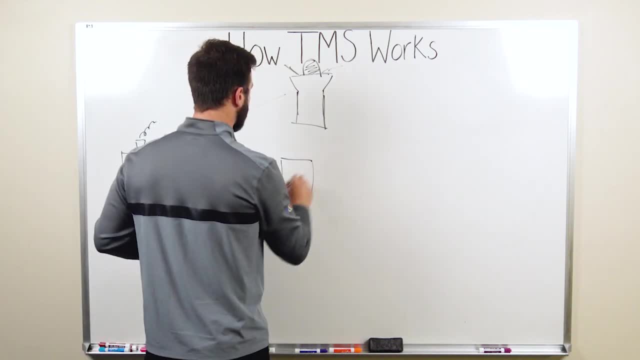 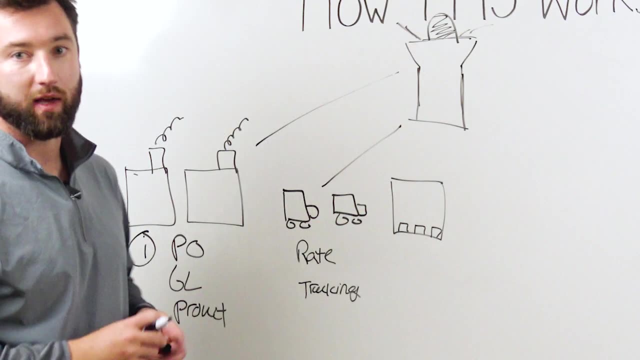 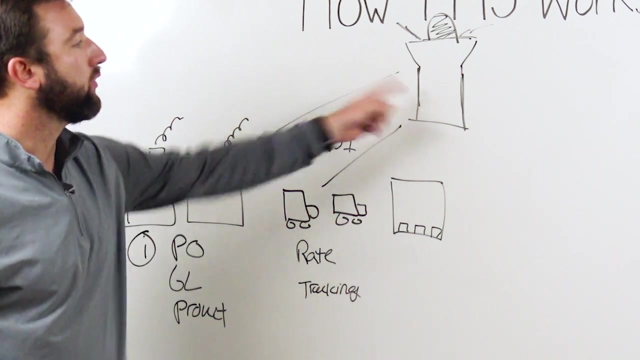 manufacturing plants to your distribution centers. you're going to want to know where they are, And so, in the right transportation management systems, with EDI or potentially API connections, you can send that information to one consolidated portal or system where you can track the movement of the goods from your 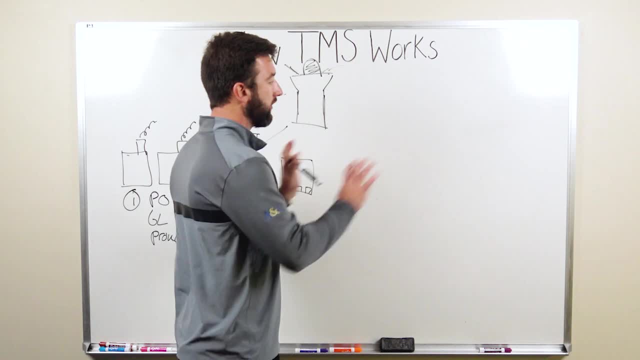 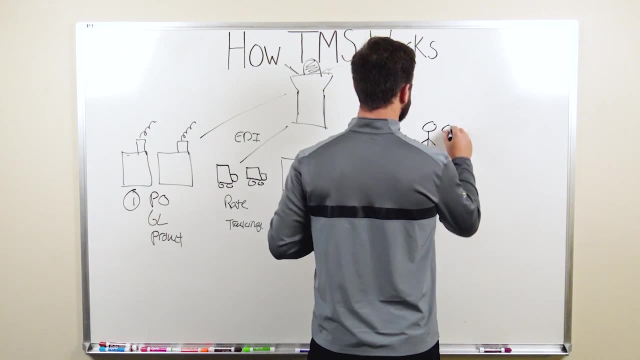 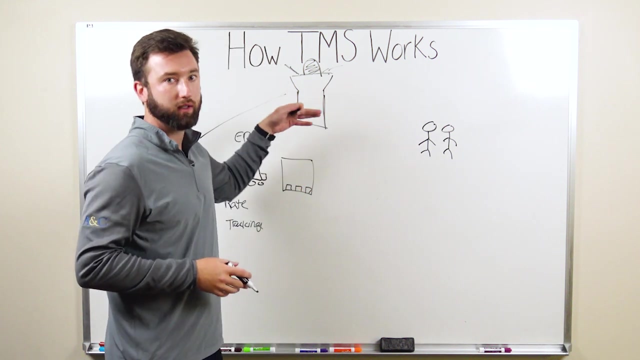 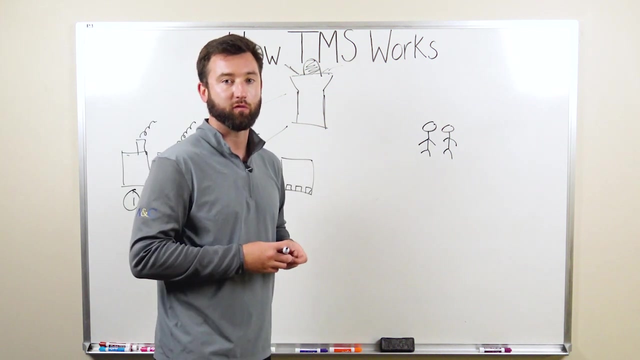 manufacturing to your distribution centers. So now, on the outbound side, we want to be able to get our product in the hands of our customers. So again, there's a bunch of different modes of transportation. Typically, it depends on the TMS that you use, So some TMS will have all sorts of capabilities in terms of the types of modes that. 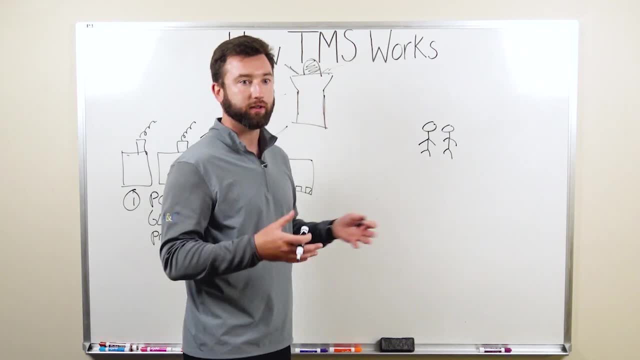 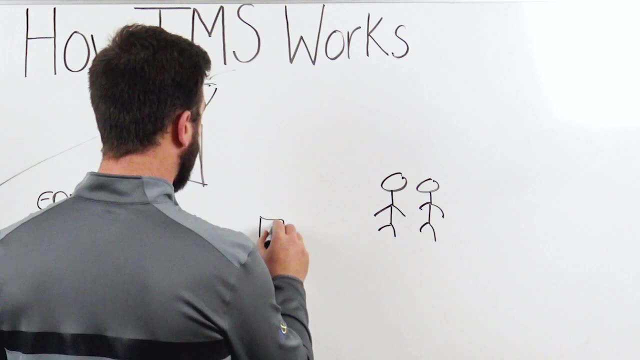 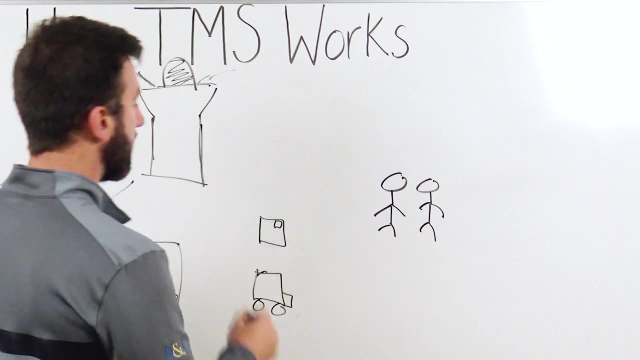 they're able to work in. Other ones might be unique to a motor shipment, like an LTL TMS or a truckload TMS, But let's pretend that we have both packages and we have trucks that are going to our end customers. So, again, what we're going to want to do is we're going to 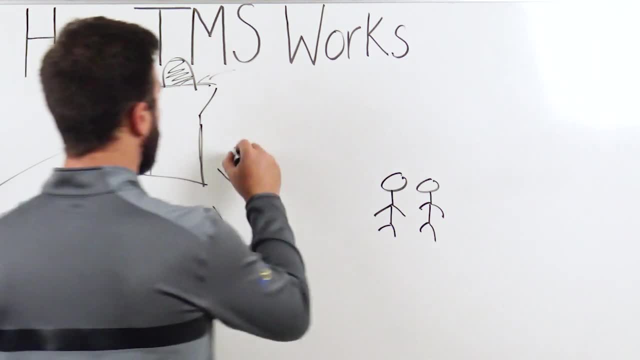 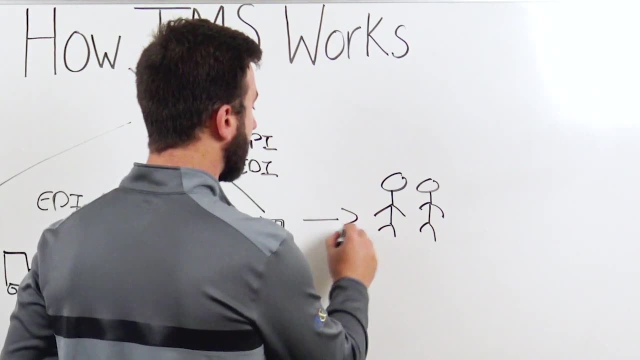 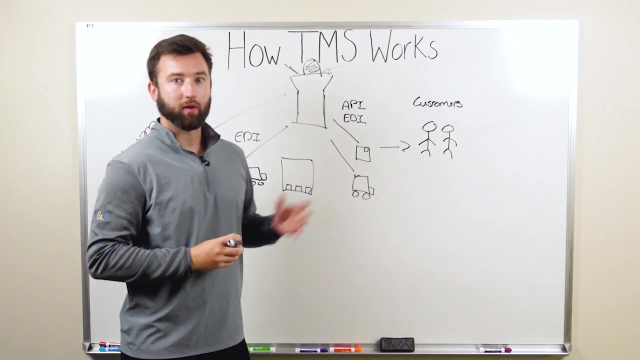 want to connect to these trucks and to these parcel carriers using API and EDI connections And we will track that all the way through our TMS blockchain to delivery to our end customers. what a lot of companies will do and most people have this experience. you know, when they say shop on amazon is those customers more and more want to understand. 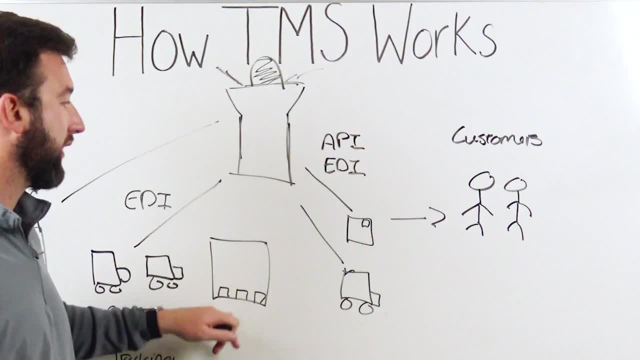 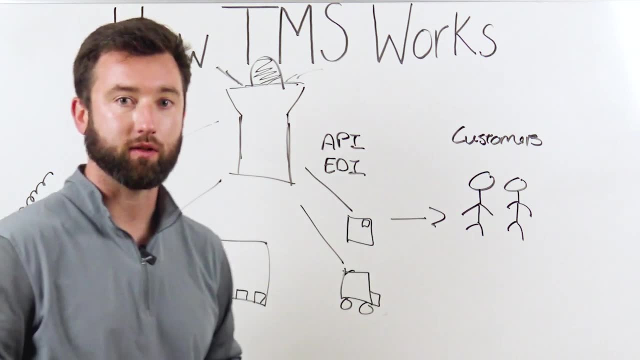 where their products are in transit. so they want to be able to track from the distribution center to the uh, through uh transport to delivery. so that's one way that you can offer an increased customer experience through a powerful system like a tms. and then one of the one of the great.